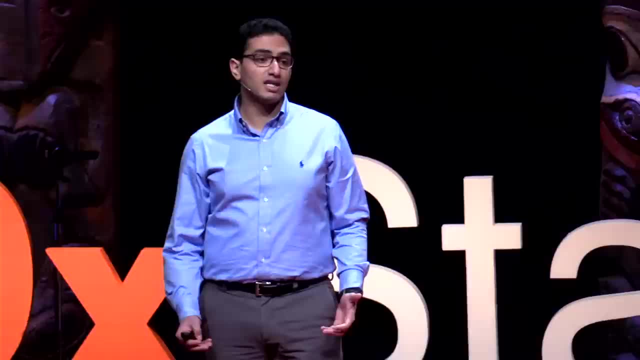 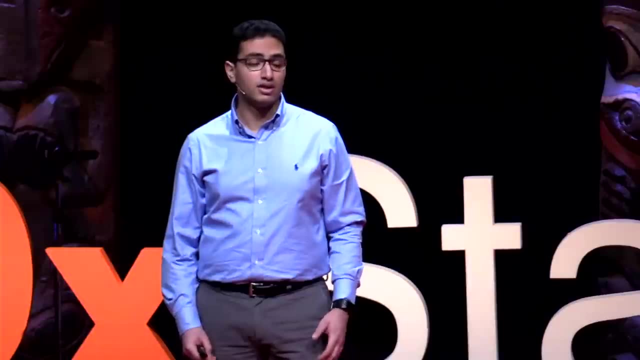 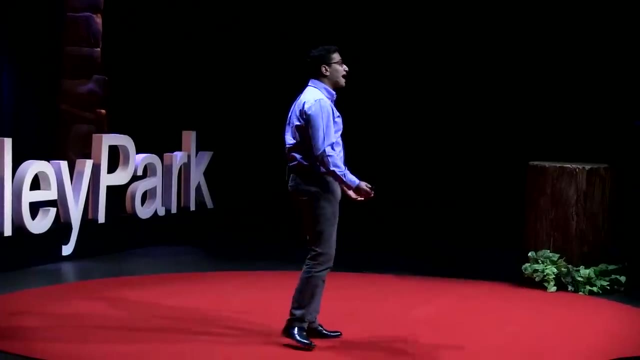 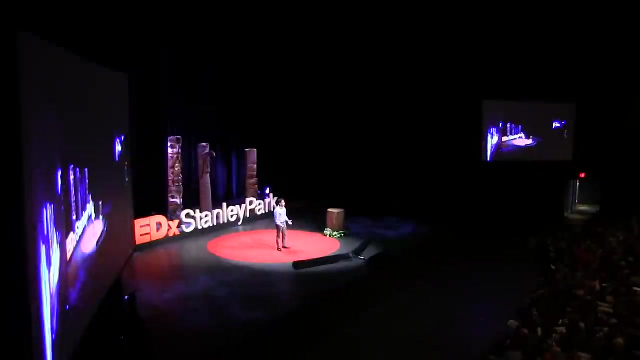 Although all the volunteers survived, the drug didn't. The devastating effects on their minds, bodies and immune systems remain unknown. These individuals may never live normal lives. Clearly, this wasn't supposed to happen, but it did So. what's going on here? While developing a safe and effective drug is a risky, time-consuming, expensive process. Did you know that it takes, on average, 12 years and 2.6 billion dollars to develop just one single drug that works in humans? Let me walk you through the process. First, drugs are tested on cells in a petri dish and on animals. Drugs that make it through this process enter human. 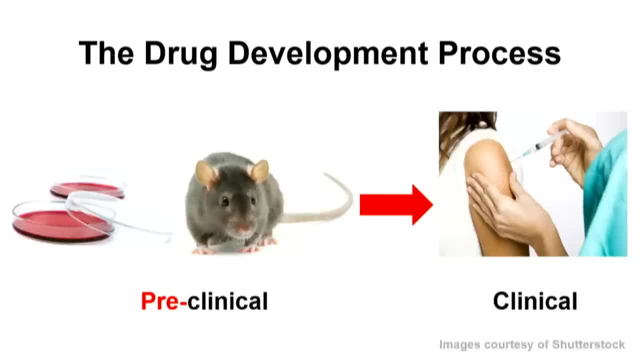 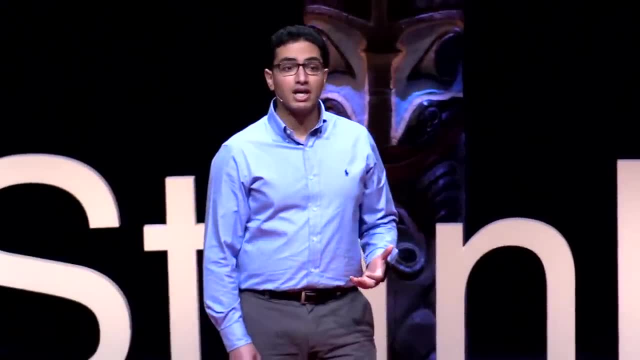 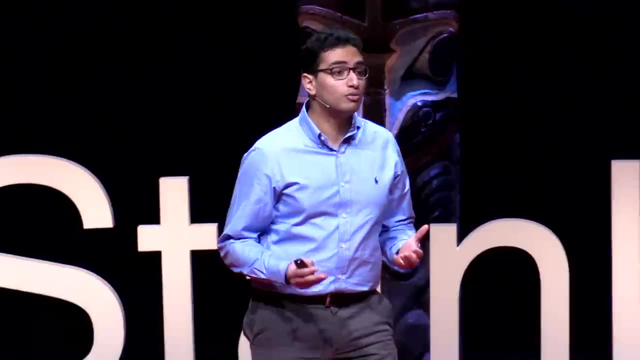 trials and only one out of ten drugs is successful. Not only is failure extremely common, it's really expensive. It costs about 200 million dollars per failed drug. If we were to double the success rate in human trials from 1 in 10 to. 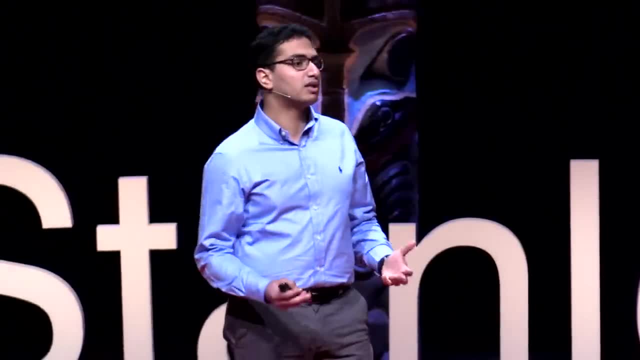 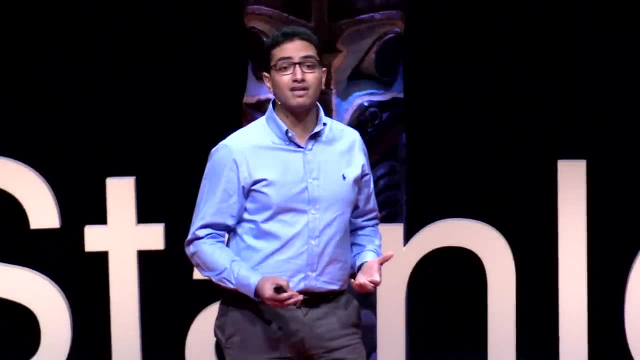 just 2 in 10,, we could save hundreds of millions of dollars. Imagine how much cheaper drugs would be for you, but, even more importantly, imagine how many more lives we could save. We can save and improve Even when a drug demonstrates that it can cure human. 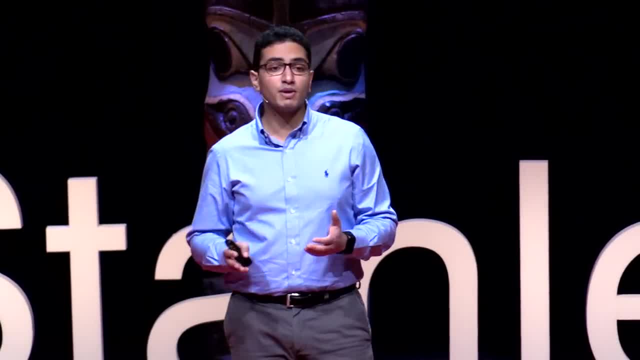 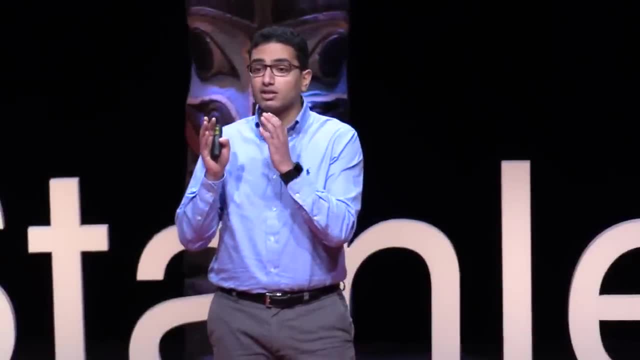 disease, it may not work for you. This is because your body is unique. A drug that will cure the person sitting right next to you might cause detrimental side effects in your body. So how do we solve this problem? You may have an idea from. 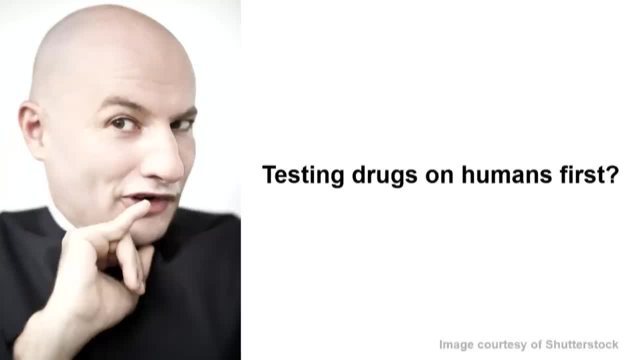 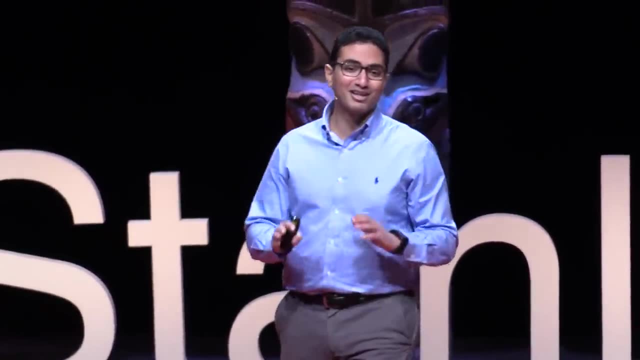 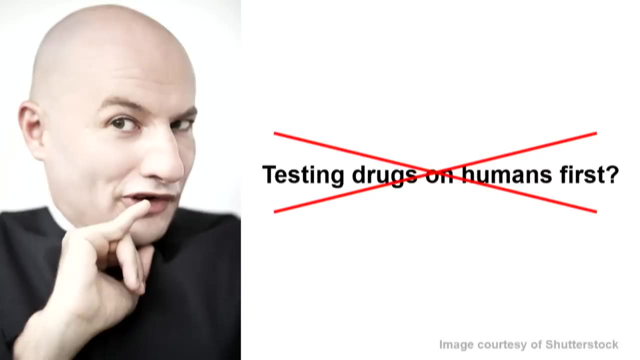 the slide. Ideally, we would start by testing drugs in humans first, but we can't do this, Or can we? No, we definitely can't start by testing experimental drugs on humans first. So what's the next best thing? What if we could engineer human tissues? 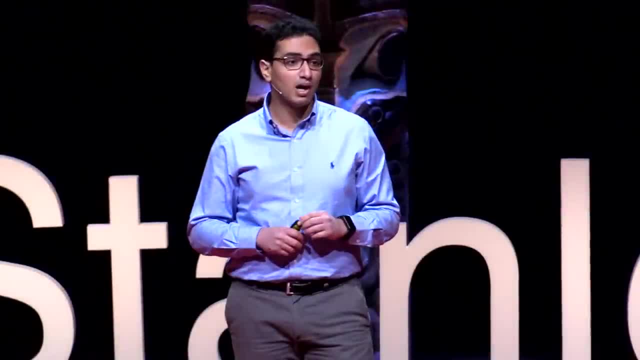 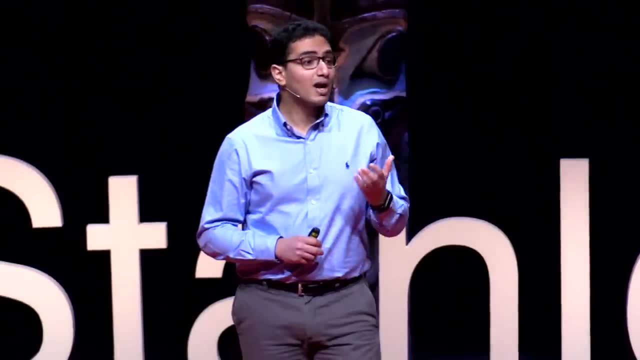 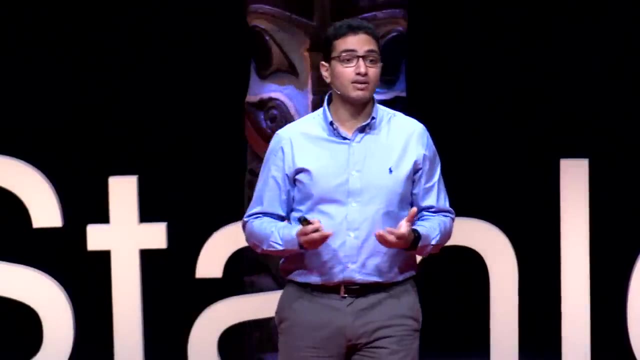 a part of a real person, but outside of their body, and test drugs on these tissues before human trials. If we can do this, we can more actually determine if a drug is safe and effective before human testing. This makes the difference. This may sound like science fiction, but I'm here to tell you today that this is already. 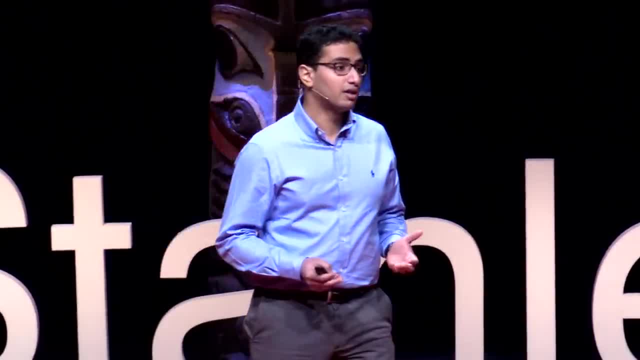 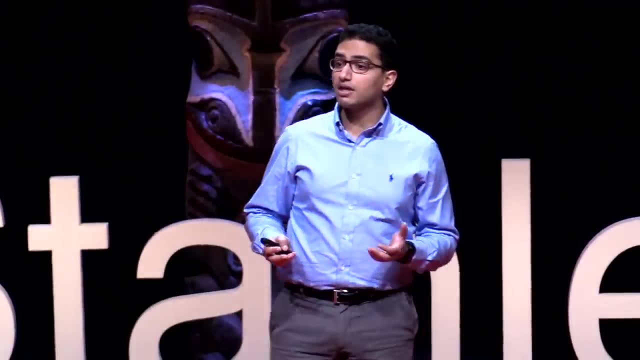 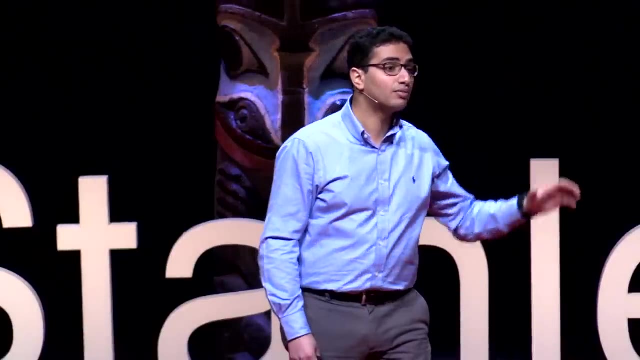 a reality Now. I'm a biomedical engineer and as far back as I can remember I've been intrigued by how things are built. When I think of engineering, I think of building things from the ground up. When I think of biology, on the other hand, I think of dissecting the human body down. 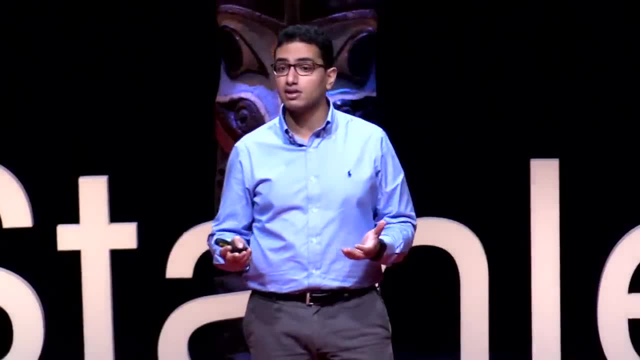 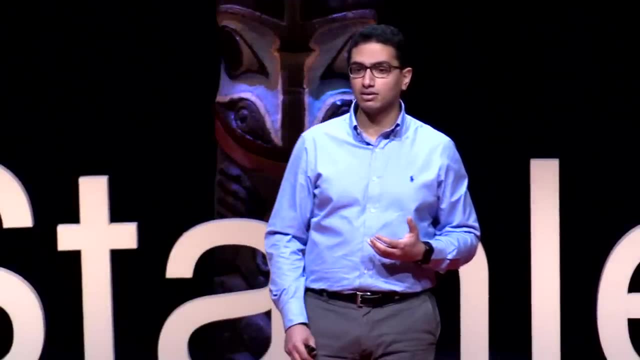 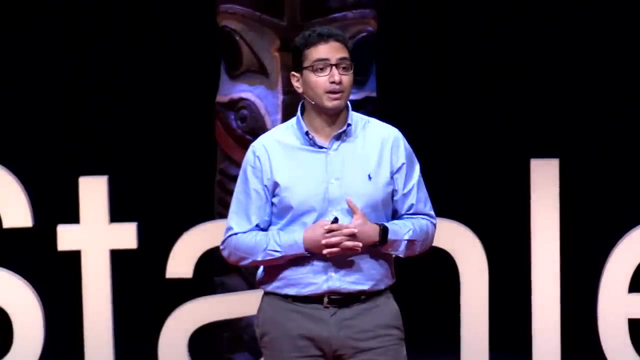 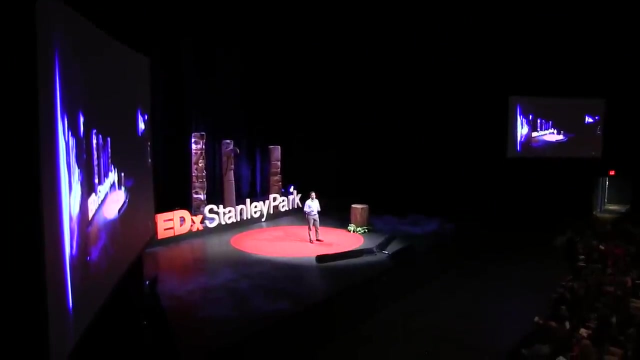 to individual cells. Think of these cells as the building blocks of your body. Our understanding of these building blocks is rapidly advancing. Biologists have taken the human body apart. Now we can combine engineering and biology to rebuild different parts of it. By combining different disciplines and collaborating, we can tackle the world's most pressing issues. 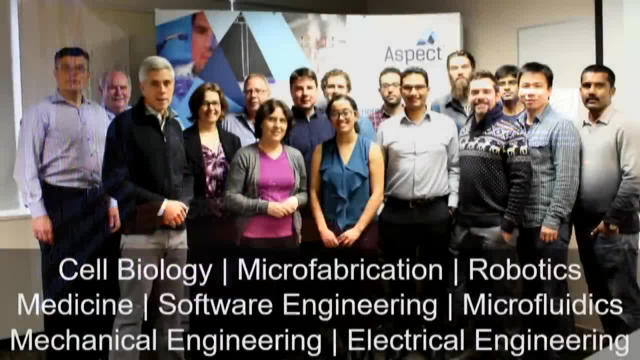 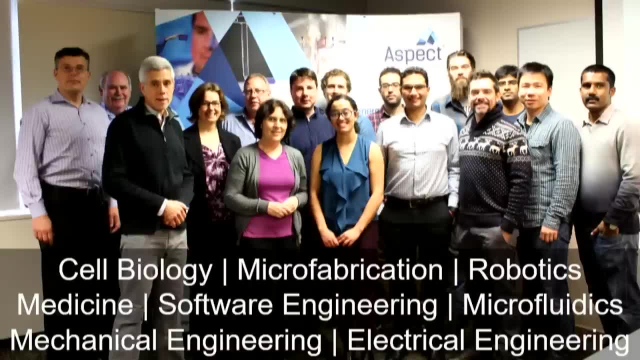 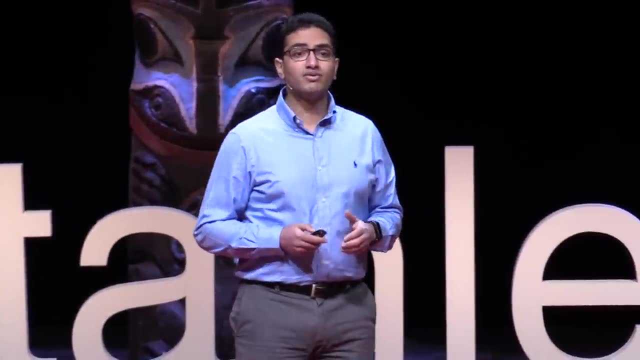 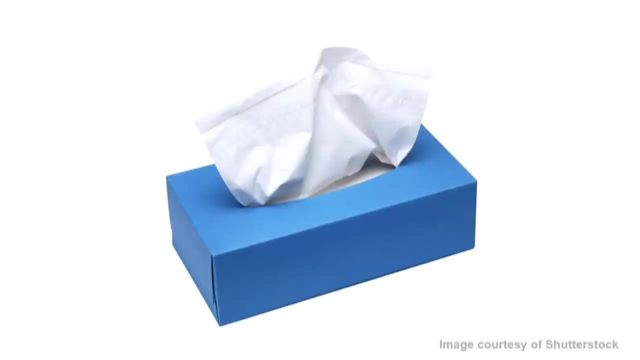 And this is precisely our story: Engineers, biologists, scientists and even clinicians all working together and collaborating under one roof to solve a big problem. This is different than each group working separately in their own silo. We've developed a 3D printing technology that could print tissues. 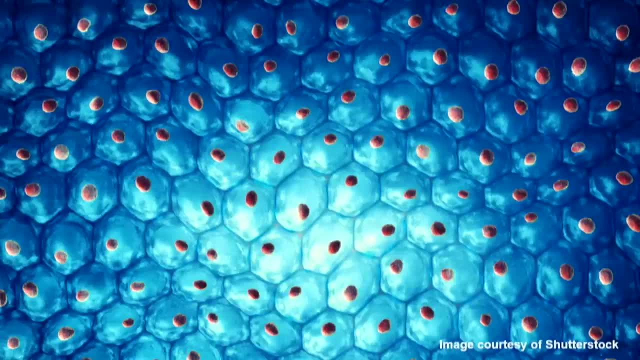 Not these types of tissues, but real, living human tissues. Here's a picture of a human tissue where each hexagonal shape is an individual cell or a building block. What if we wanted to print a part of a lung, An airway, for example? 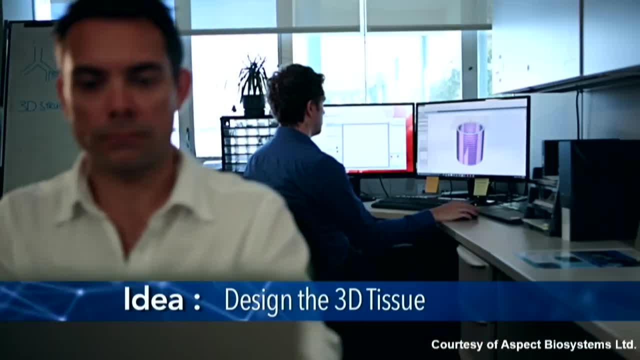 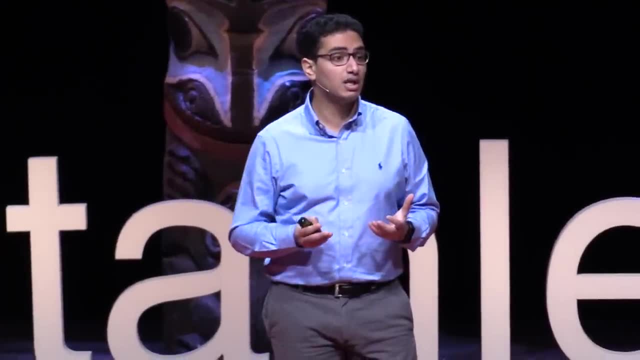 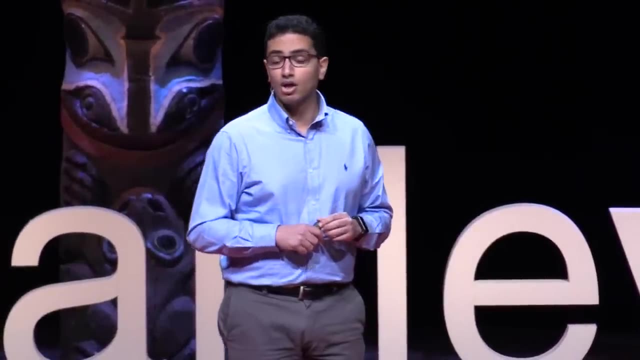 Well, we'd start out by designing a 3D computer model of an airway. This model would then be printed layer by layer using a machine called a 3D bioprinter, Instead of using plastics and other non-living materials used in standard 3D printing. we 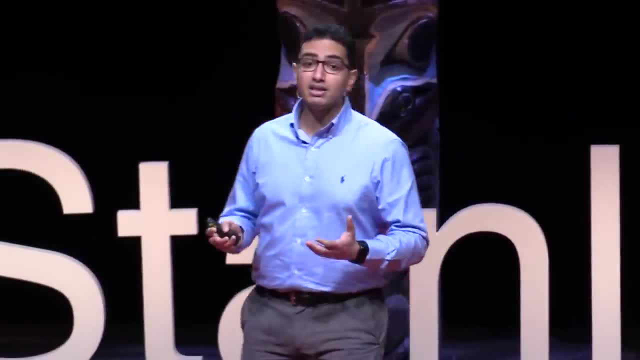 use real living human cells. We combine these cells with scaffolds to provide a suitable and comfortable environment for our cells to grow. The cellular materials then become our inks. 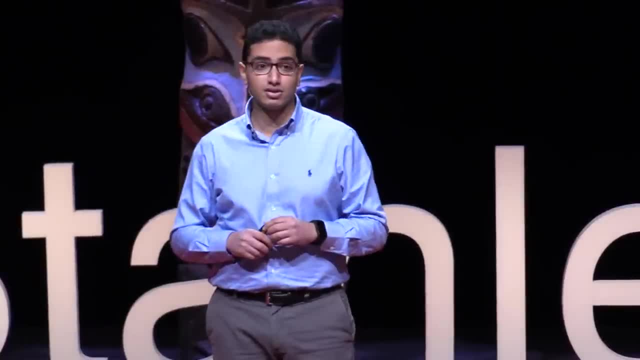 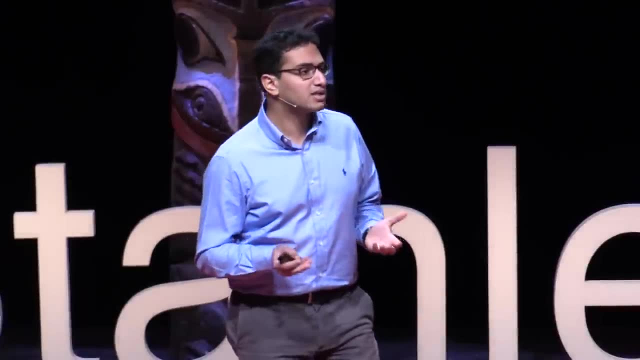 Kind of like the inks we use in conventional desktop printers. We now have our building blocks and are ready to construct our tissue. So how do we deposit these living inks? Because tissues are composed of many different building blocks, we need to handle many different. 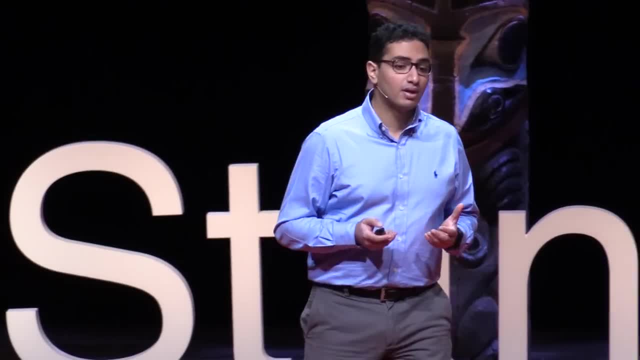 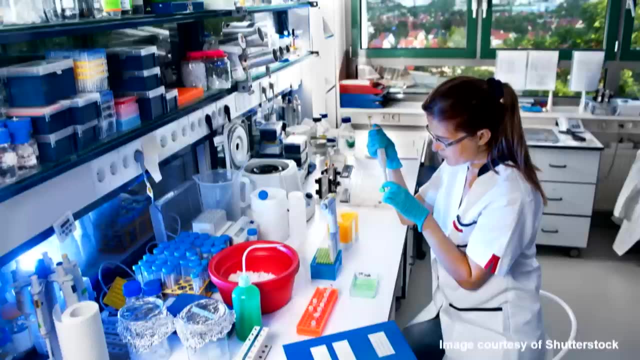 materials at once. You may be thinking of a lab that is filled with biologists manually mixing and preparing different cells and biomaterials, and they would be doing a lot of adjustments to typical cells- this by hand. They would need access to different dispensers and the ability to switch between 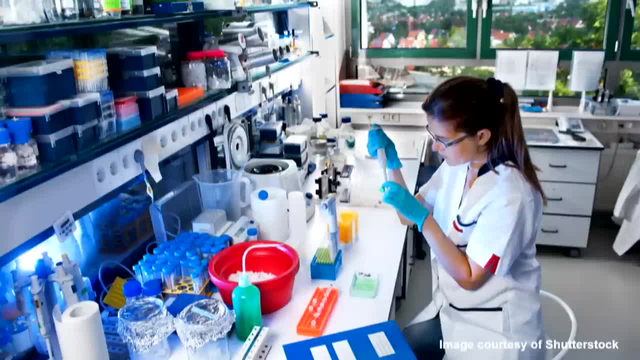 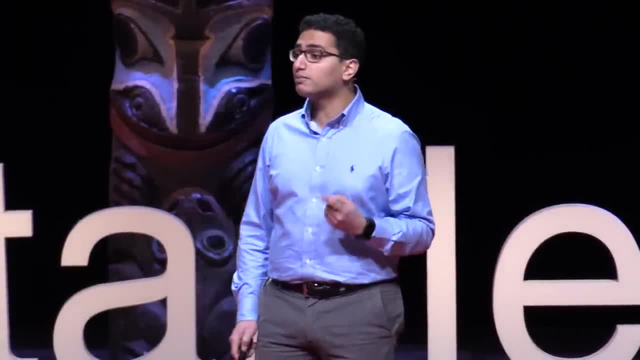 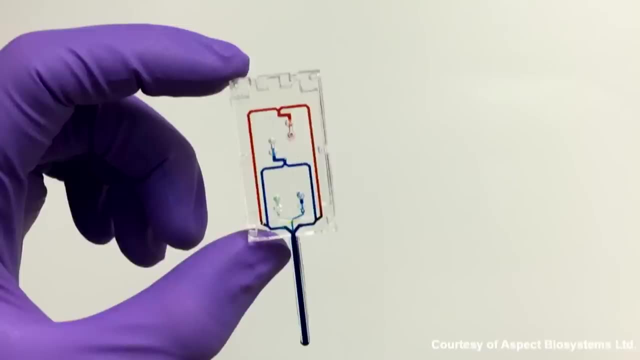 these dispensers throughout the process. This would be slow and manual. What if we could integrate and automate many of these lab functions and shrink them down to one simple chip? We call this chip lab on a printer. I brought one with me today and I'm holding one in my 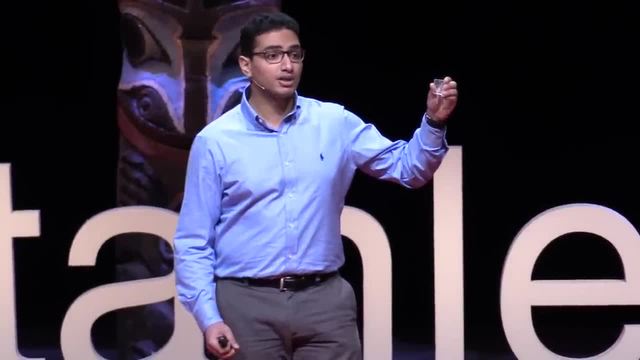 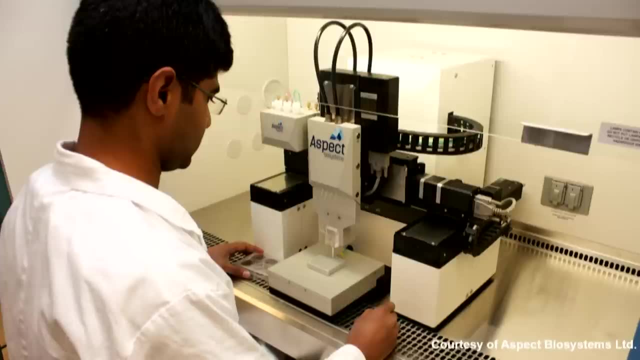 hand. right now, Our 3D bioprinter uses this lab on a printer to deposit living inks. Our lab on a printer allows us to take multiple living inks and deposit combinations of these on the fly through a single nozzle to rapidly develop living structures. Here's an example. 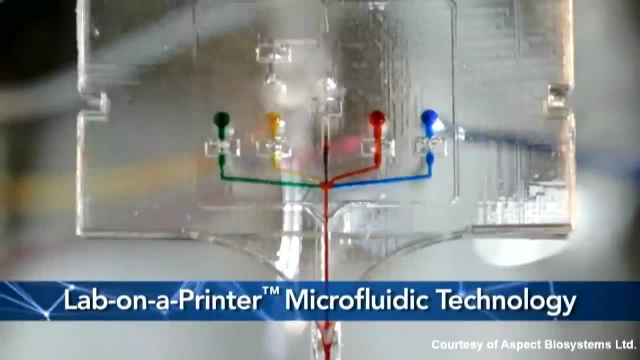 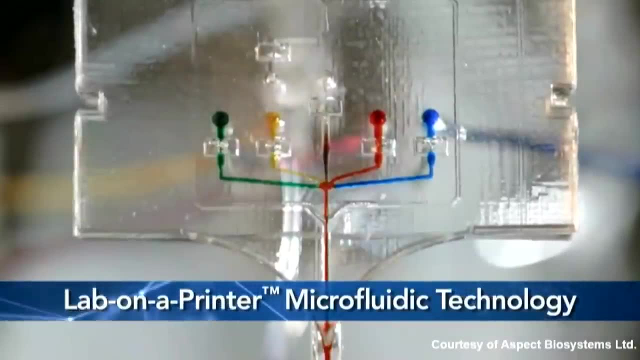 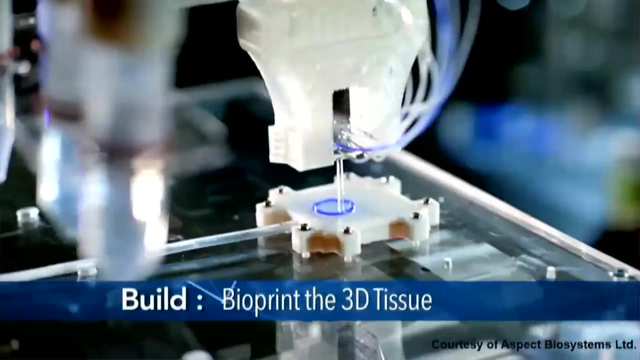 where our lab on a printer is depositing many different materials at once: The blue, red, yellow and green materials. well, these could represent different cell types, different growths. Our lab on a printer then deposits these living inks layer by layer, to construct a 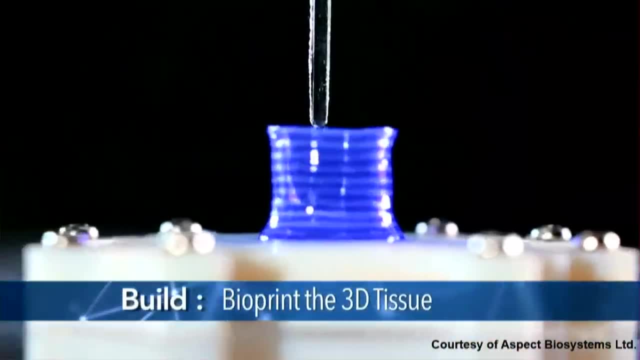 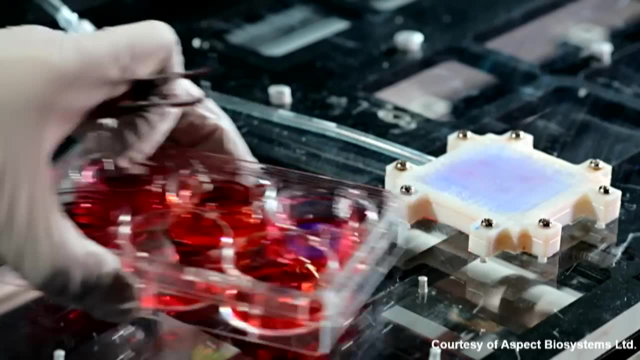 living structure. This structure could be an example of an airway or a blood vessel. Immediately after printing, these tissues are put into an incubator, which recreates the conditions inside of our body. If we were to zoom into one of these printed structures, 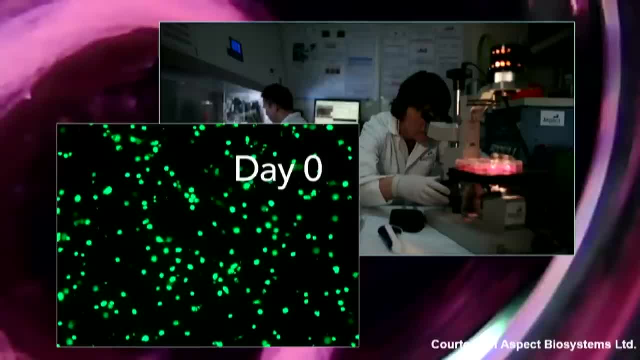 immediately after printing, we would see many different structures. One of these printed structures is a cell. As many of you have seen, at the top you can see many green dots. Each one of these dots is a cell. Here's how they look after a couple. 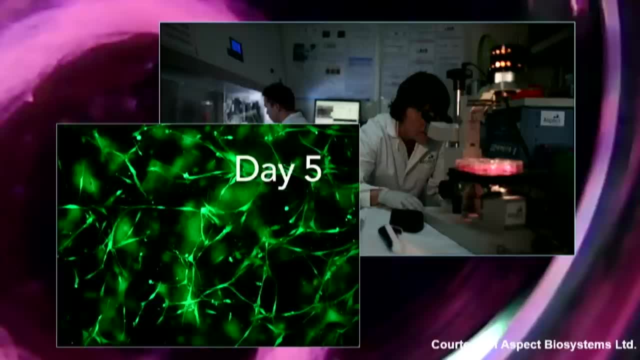 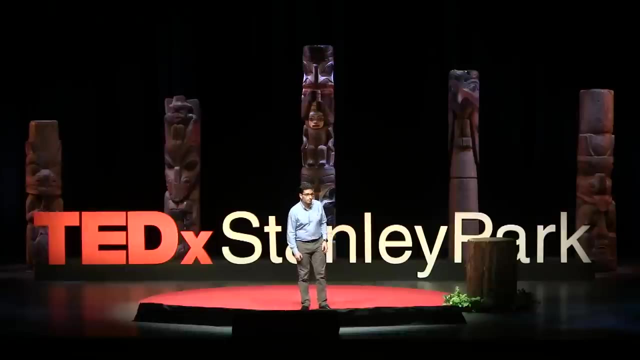 of days, Because we provided a suitable and comfortable environment for our cells to grow, they begin to talk and form interconnected networks. Our 3D printed structure has transformed into human tissue. As individuals, we are all different – and the diseases that affect. 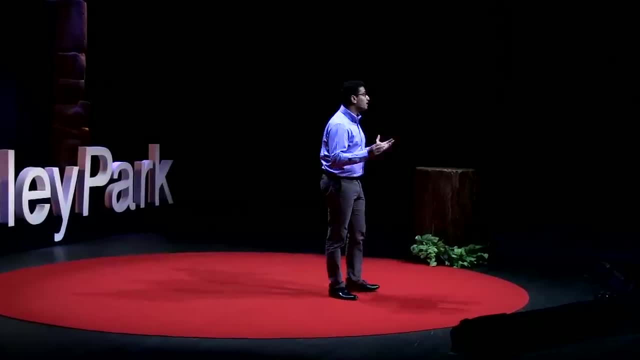 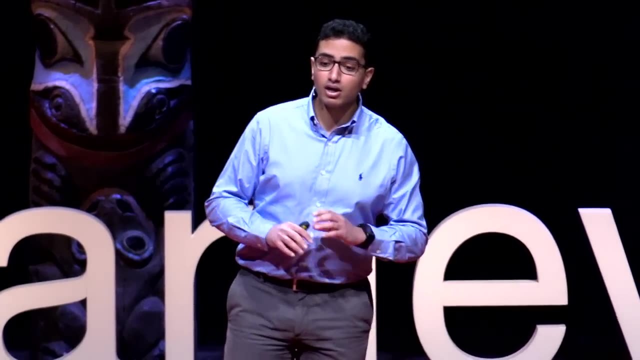 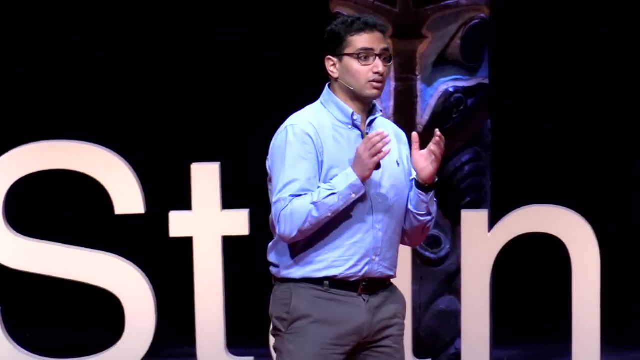 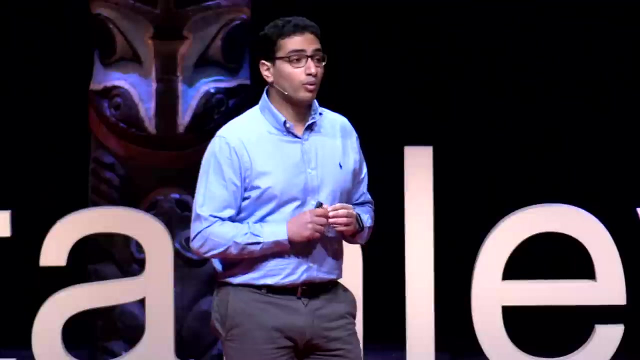 affect us in different ways. This is true for many diseases, including asthma, cancer and other diseases. Now our goal is to develop an entire replacement organ that could replace a diseased organ inside of your body. We're several years away from this, but what could we do today? Well, we could print smaller. 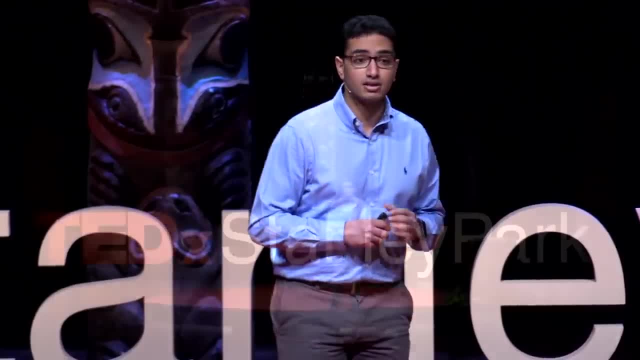 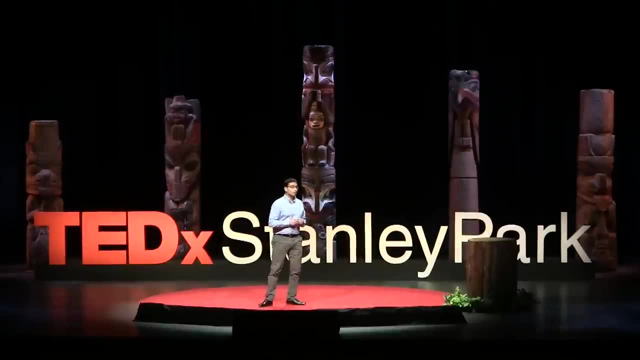 parts of organs and use these tissues to test drugs and test the diseases that we suffer from and develop drugs and cures for these diseases. For example, we took muscle cells from a donor lung to construct an airway. We took these cells and we printed them into tubular structures similar to the one that I 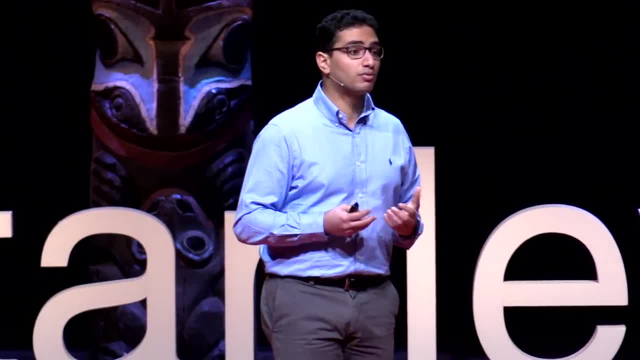 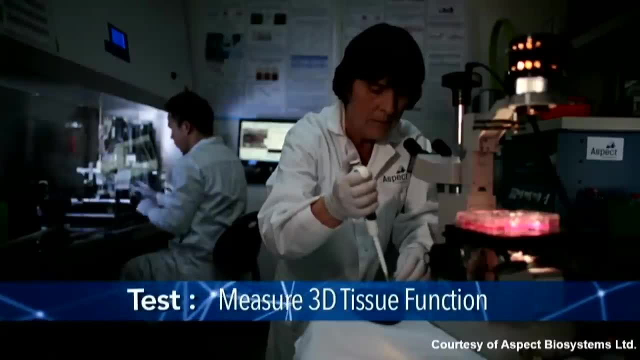 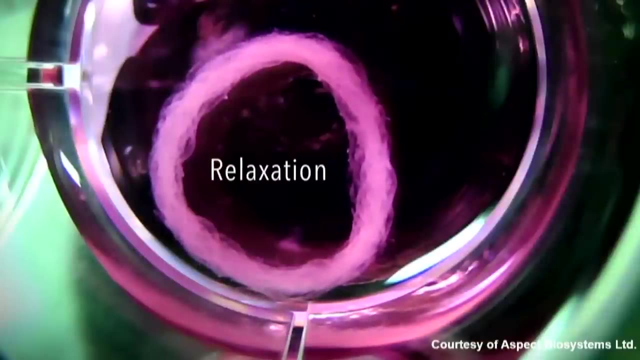 showed you Now. during a real-life asthma attack, our body releases a compound called histamine. This triggers the smooth muscle tissue inside of our airways to contract. We dosed our bioprinted airways with histamine and they began to contract. We recreated an asthma attack outside of the body. We 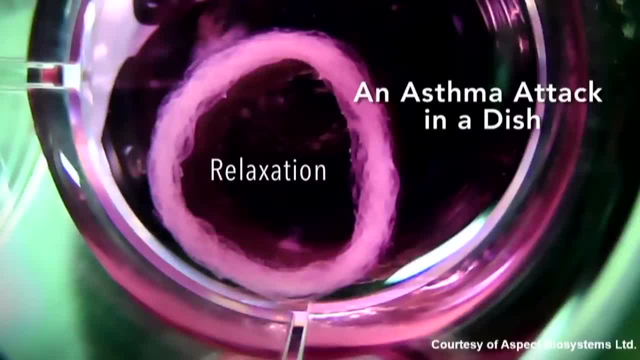 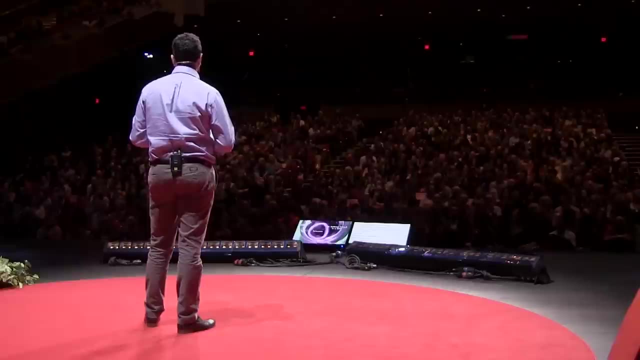 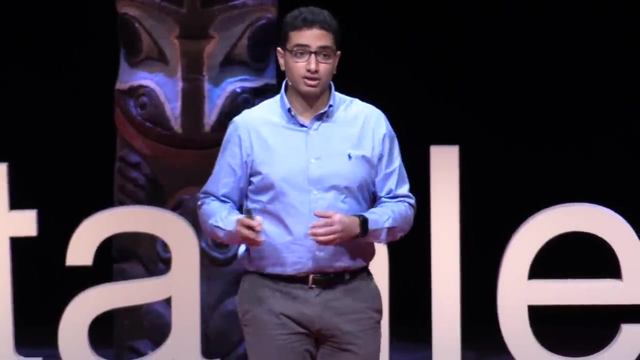 then dosed our bioprinted airways with a common anti-asthma drug used in inhalers, and they began to relax just like the airways of an asthmatic patient. So where are we going with all of this? Well, I showed you one application of 3d. 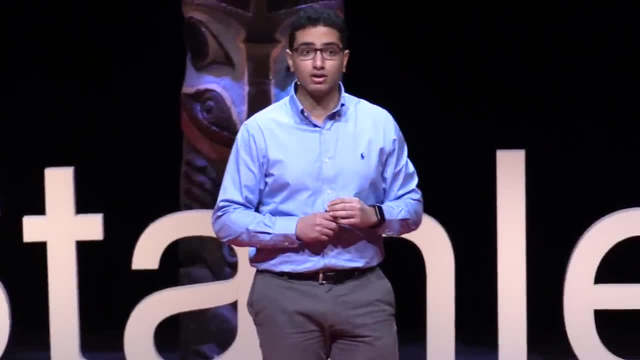 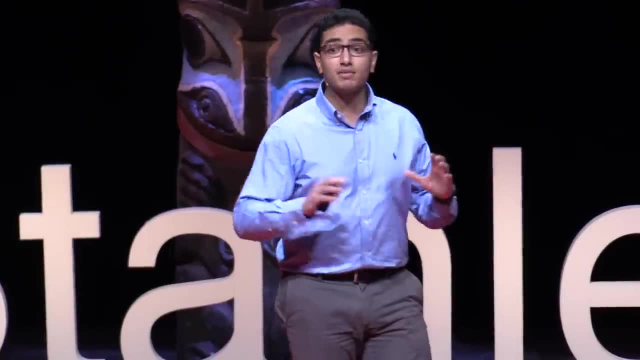 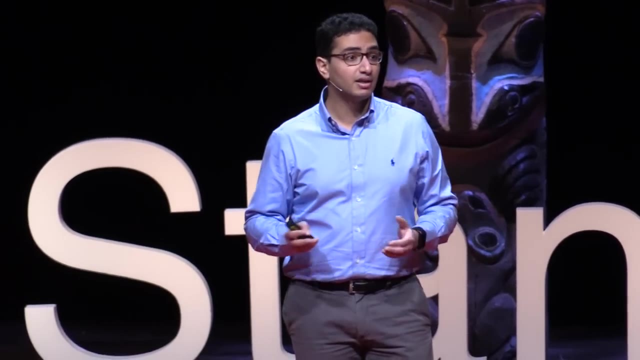 bioprinting, that is, in the near future. Where are we planning to take this technology? My vision for this technology is that we could one day create entire replacement organs. Just imagine no organ waitlist. A doctor would simply take cells, perhaps from your blood. These would be taken to a lab and reprogrammed. 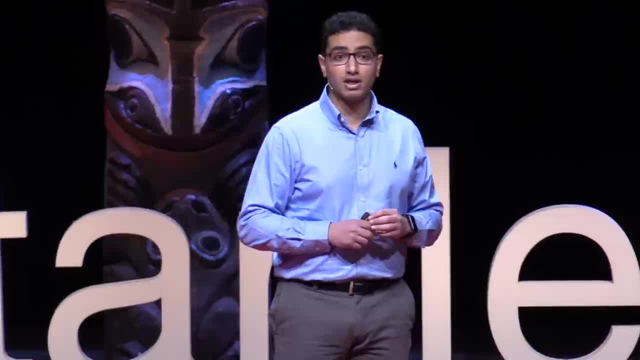 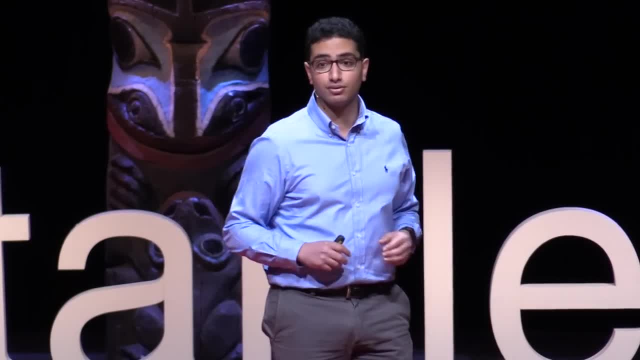 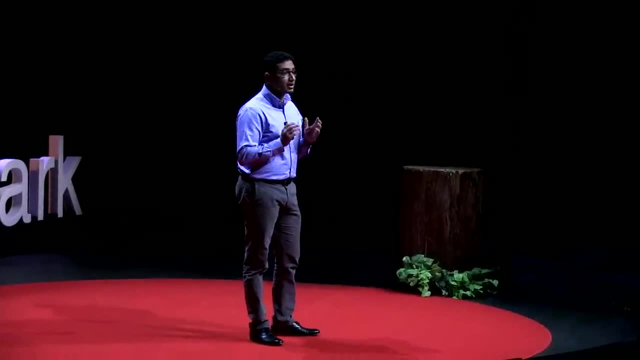 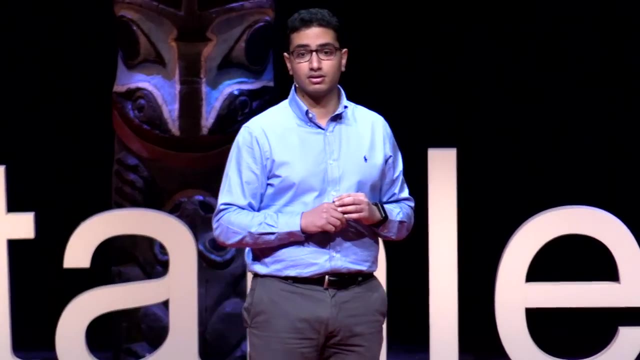 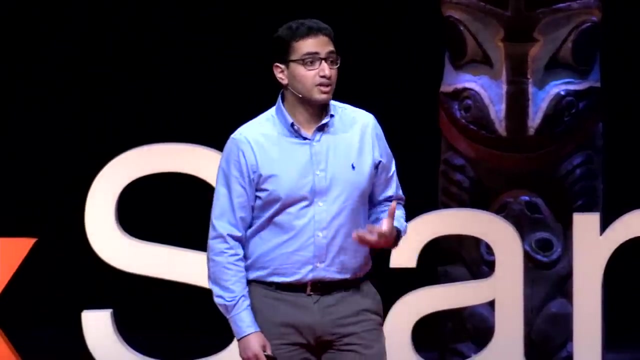 we would construct an entire organ just for you. This organ would be made up of your own cells- just think of that- your own building blocks. so no chance of rejection. Bioprinting will enable us to accurately determine the human response to drugs. What this means is that we could eliminate drugs that won't work in.